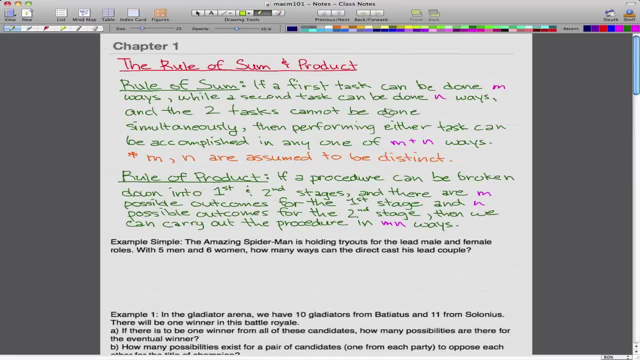 a second task can be done n ways and the two tasks cannot be done simultaneously, then performing either task can be accomplished in any one of m plus n ways, And m and n are assumed to be distinct. So what the? the rules here is that the two tasks? what the fuck? 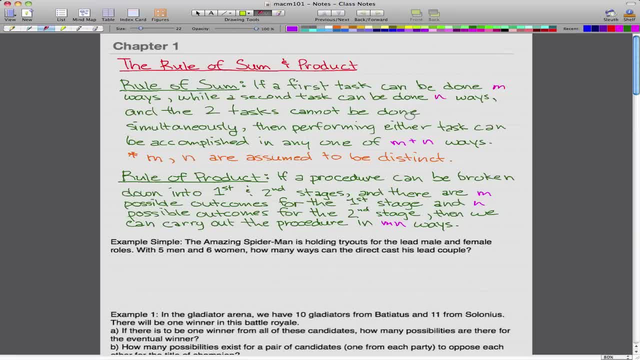 is- oh sorry, I swore So the two tasks cannot be done simultaneously, And then by performing each either task. this can be accomplished in m m plus n ways. So that's pretty simple, And we'll go through a couple of examples to make sure you really 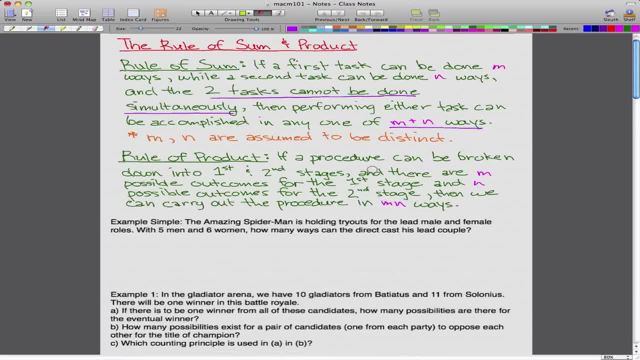 get it. The second part is the rule of product. If a procedure can be broken down into first and second stages and there are m possible outcomes for the first stage and n? n possible outcomes for the second stage, then we can carry out the procedure in m mn ways. So 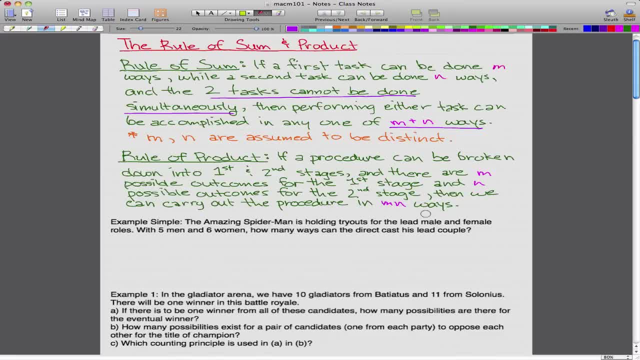 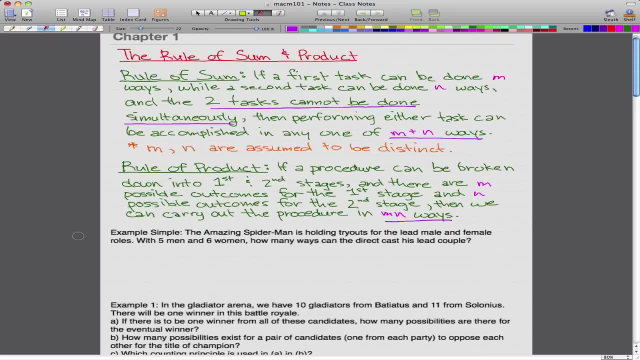 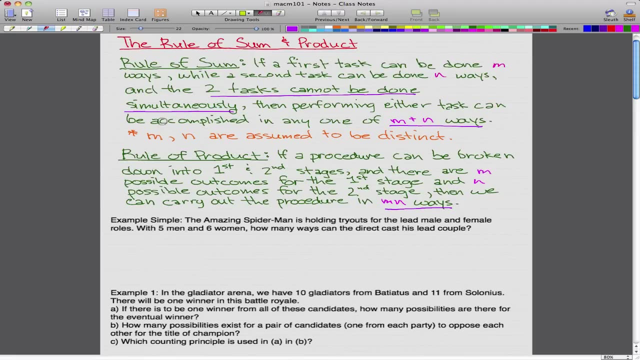 right. mn is m times n, And that's the amount of ways that we can handle it, handle this for a rule of product. So these are rules and they are pretty damn abstract, Like if you just ask me to explain this to you. I got this from a book. I don't even know what it means, But then I really. 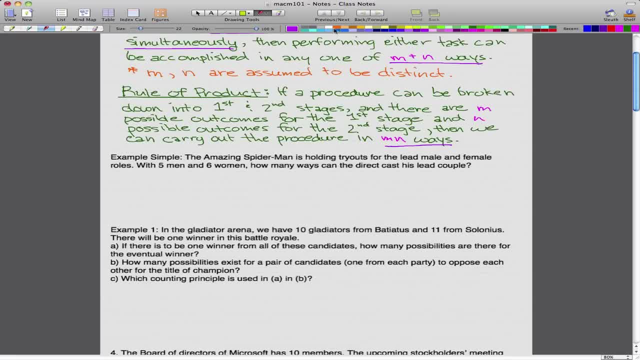 understand how, the, how, the, how the questions work, And that's all you guys are really here to know about, to learn about, I guess. So here's a simple example- And I pretty much made this or modified it- from the book that I'm using, which is from Grimaldi: The Screen. 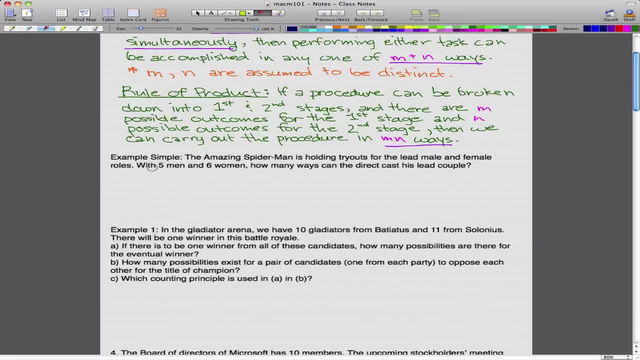 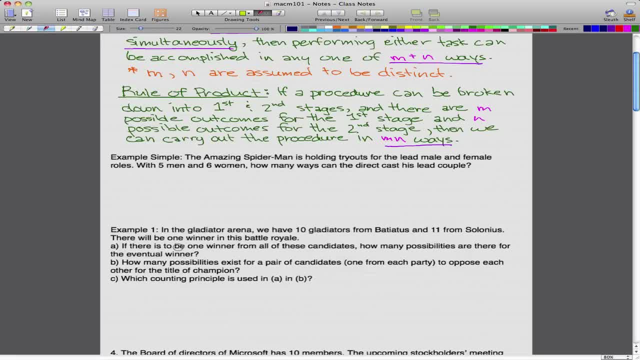 movie that's out at the time of the making of this video is holding try-outs for the lead male and female roles, And there are five men and six women. How many ways can the director cast his lead role Or his lead couple? God dammit, I gotta, I gotta, edit. 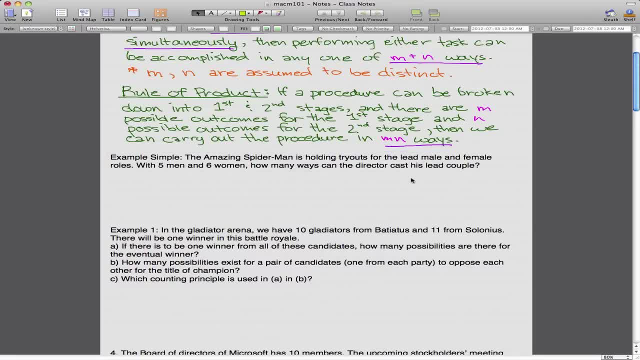 this A little bit of OCD: cast this lead couple. so it's really simple here and this shows the rule of rule of product. so it's pretty much just 5 times 6 and that's 30. so there's 30 ways that. 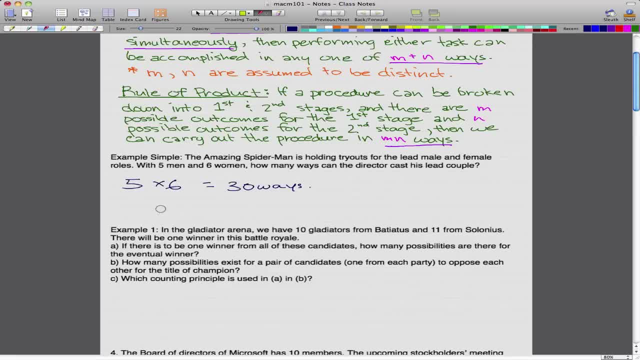 director can cast as the couple. why? well, because we have five men and six women. so, to show you in a diagram, we have one, two, three, four, five men and one, two, five, six couple. now, one of these men can be connected to any one of these six. 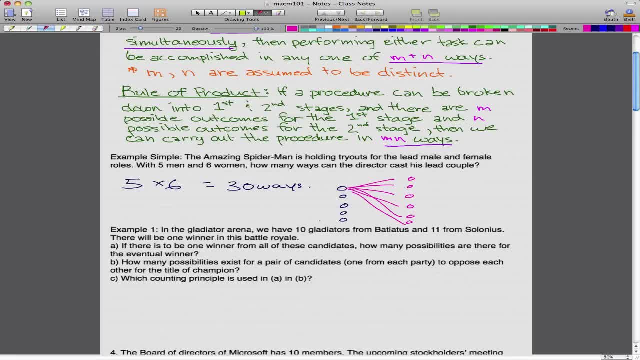 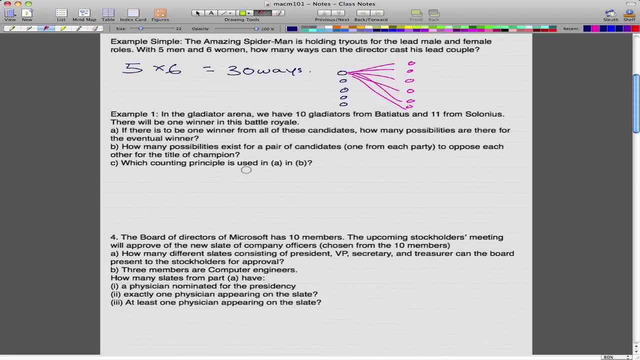 women, and so can the second guy and third guy, in the fourth guy, in the fifth guy. so taking five and and each five guys can have six possibilities to to connect with a different female, then that gives us 30 ways, simple example, and I think I explained it well enough that you'll get it. 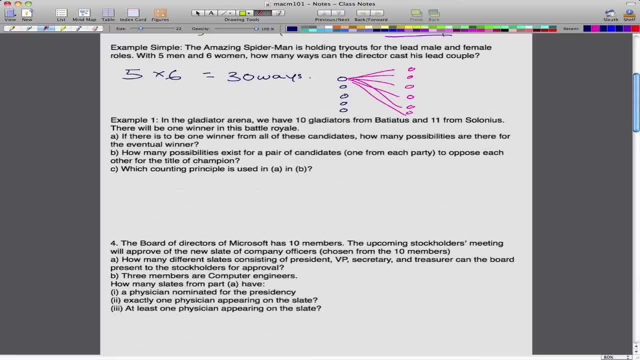 so so example one: in the gladiator arena we have 10 gladiators from body artists and 11 from Salonius. yes, I am highly addicted to fucking Spartacus. that's best series I've seen so far other than Game of Thrones. Game of Thrones is also. 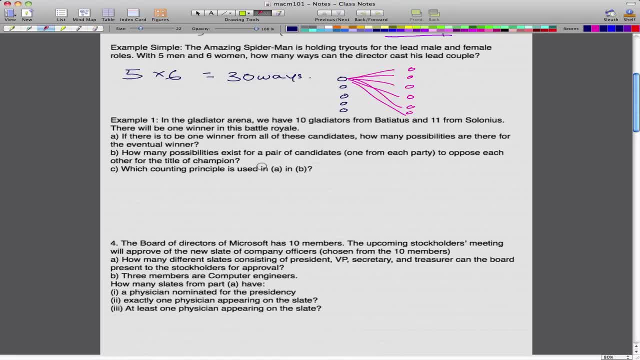 dope. so there will be one winner in this battle royale. and here's the first question: if there is to be one winner from all these candidates, how many possibilities are there to be one winner from all these candidates? how many possibilities are there for the event, for the eventual winner? so we have ten gladiators from body. 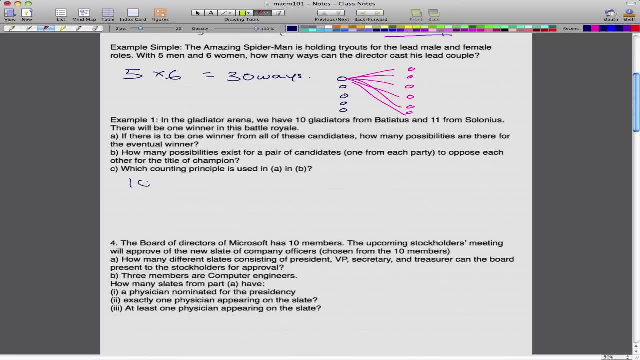 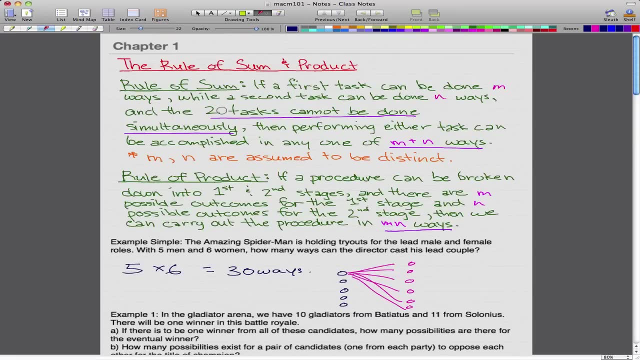 artists. so that would be 10 from B and an 11 from Salonius for them from Salonius. so this is an example of the rule of sum because, as you can see here, there there two things that cannot be on the same team. pretty much we have ten people from. will body artists team and ten people from both of the Dentist andух, and I'm going to go ahead and pass on material in the other undo clip and it's because it's good job. if you did it, you'll win if you're not paying any benefits. 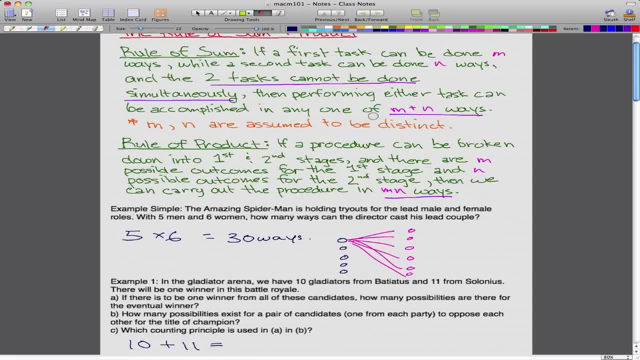 ready to take anything. you went- okay, I'm excited- the next part let me show you. okay, let's go ahead, let me do it, go ahead and do it and I'm going to go ahead. and 11 people from Saloni's team. so there's- there's 21 different people, so of 21, 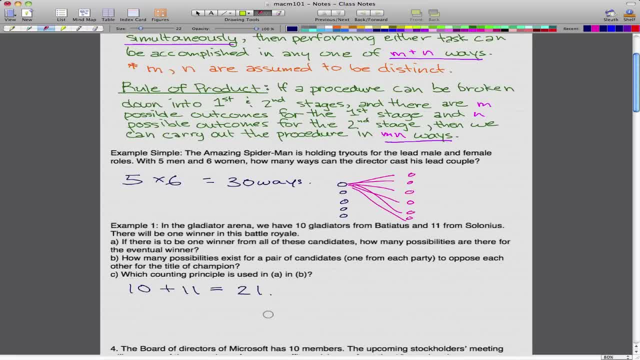 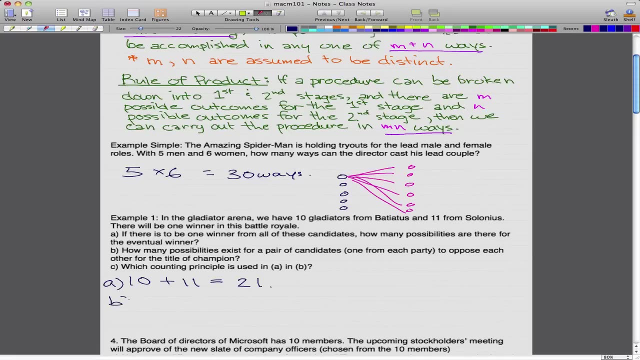 different people. if each of them are just gonna kill each other, then pretty much for the eventual winner, there can be one winner and there could be 20 different ways, because there are 21 different individuals that can win. so that's a and B is how many possibilities exist for a pair of candidates, one from 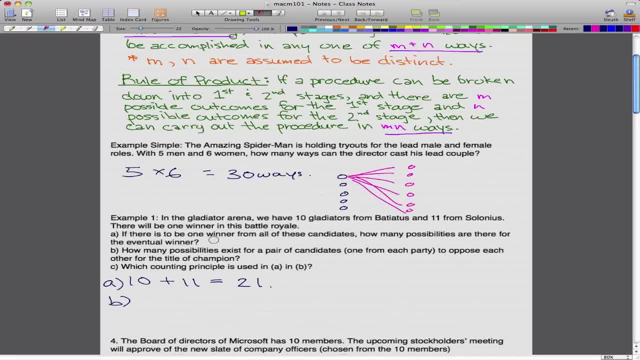 each party to oppose each other for the title champion. so pretty much this is: if you have guess rule a product, then you guess. right, you have 10 people from body artists and 11 people from Saloni is similar to this, similar to this. we have like say, say this: I have 10 circles here in 11 circles here, the put the. 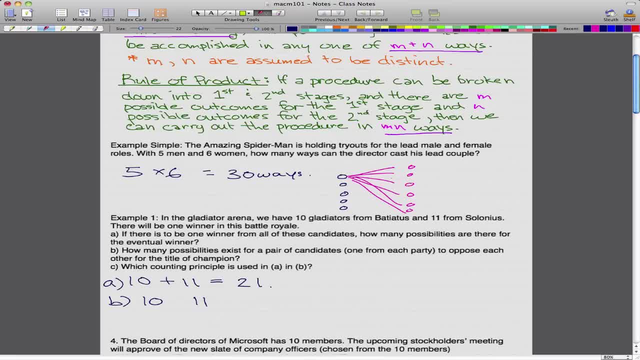 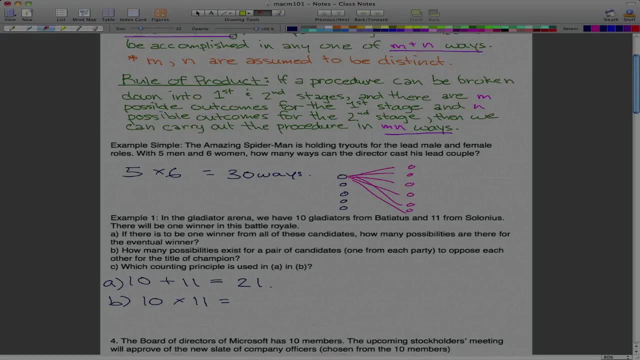 first person can can be peered against any of the any of the other 11 from the opposing team and so on, and that's what. that is what gives us 110, 10 times 11. god, I have horrible mental math, so in this case I'm just gonna freaking news calculator. so we have 110. my brain is. 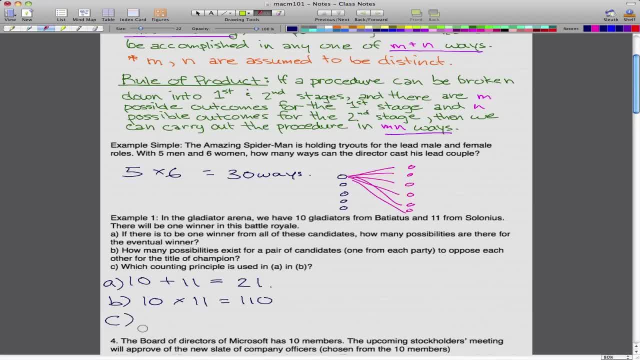 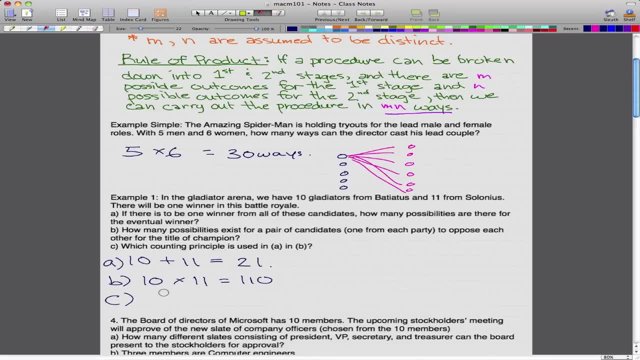 just not working today. that is my excuse for my horrible math. but then I somehow got it in the course two things. it's just fucked up. so see which counting principle is used in a and in B. so in a, the rule of sum and in B, B it's the rule. 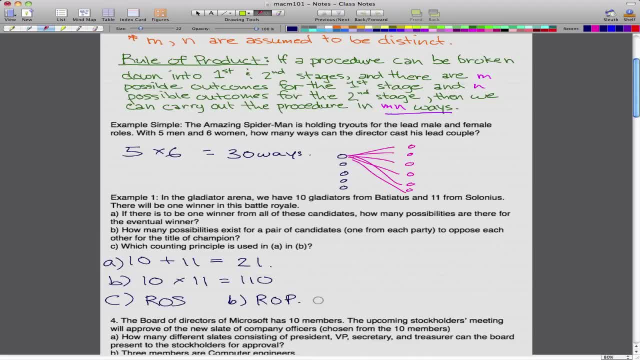 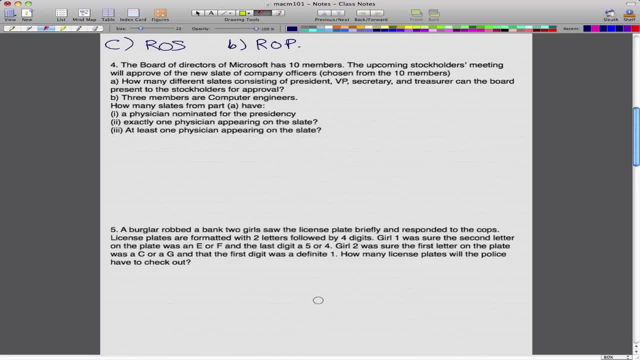 of product. so here are. here are two more examples that I'll go to in the next video. I'm gonna stop here. so you guys know that I'm gonna stop here. so you guys know that I'm gonna stop here. so you guys know that I'm gonna stop here. so you guys. 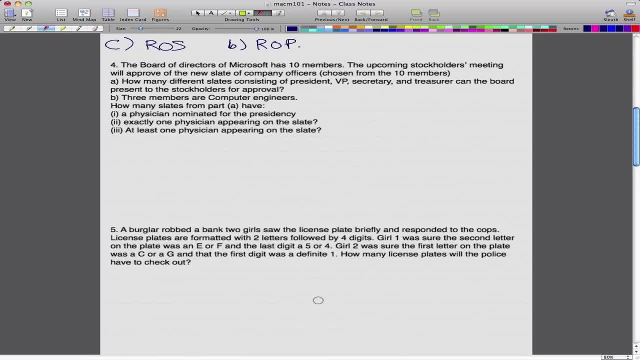 can take a look. look at this, exact these examples and try to get them on yourself in the next video. we'll go. we just go through it and do these two examples and we'll call it. I will call that that. other than that, please rate comment, subscribe, if you haven't already follow us on Twitter and like us on.